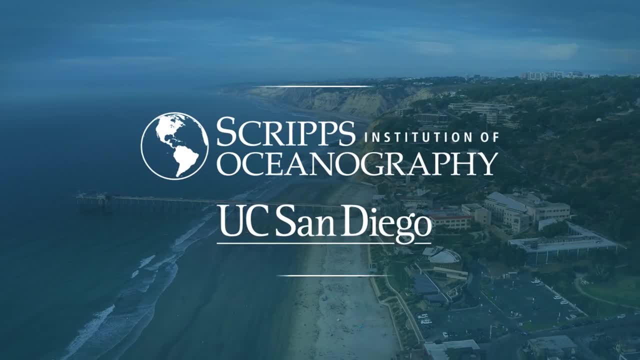 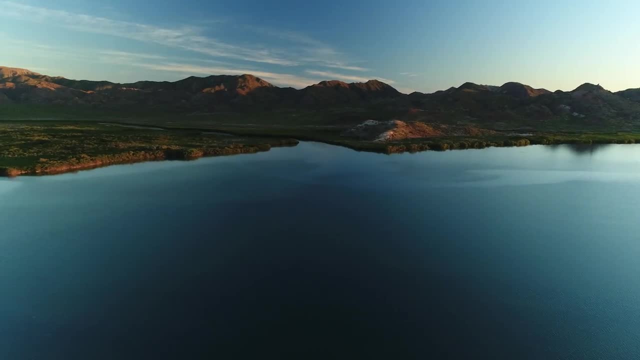 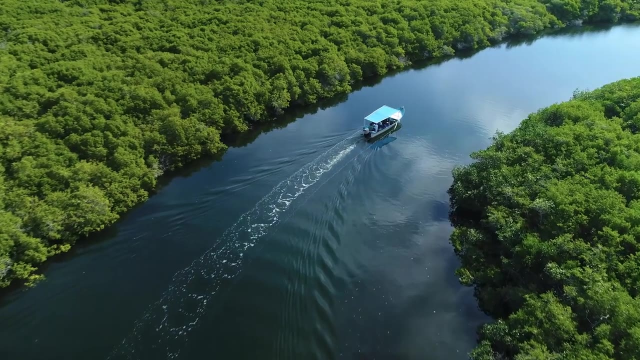 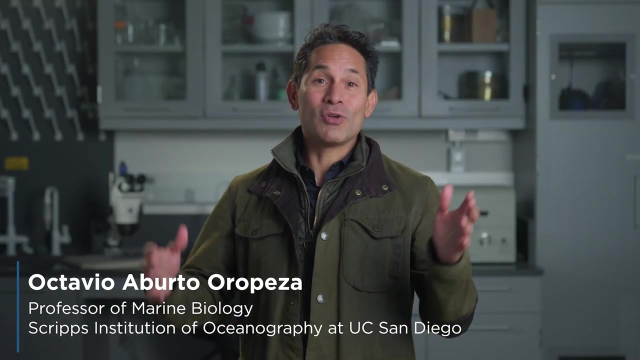 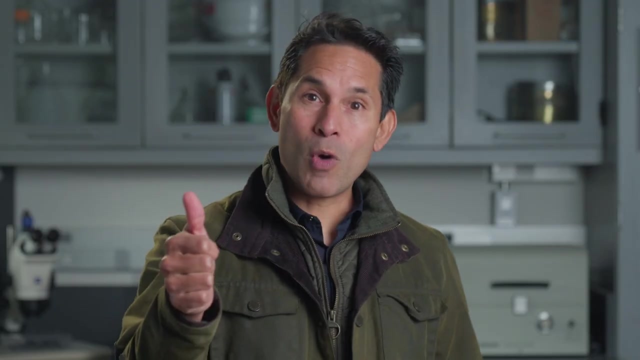 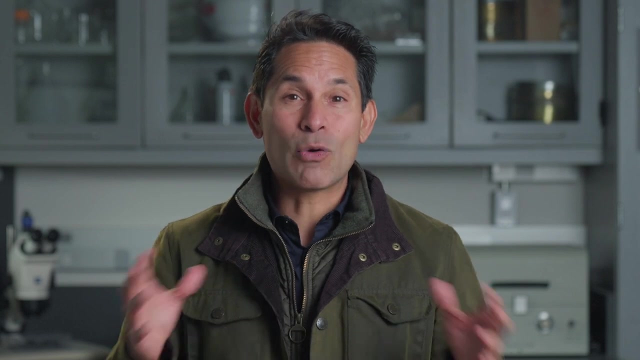 Mangroves are one of the most impressive ecosystems on the planet. They interface the ocean and the land, forming a thin line of trees that protect the coast areas much like our skin protects us. They not only provide us protection against hurricanes or erosion. they provide us with many other ecosystem services. They purify the water by filtering it through the sediments, provide nurseries for fish and other species and sequester carbon. 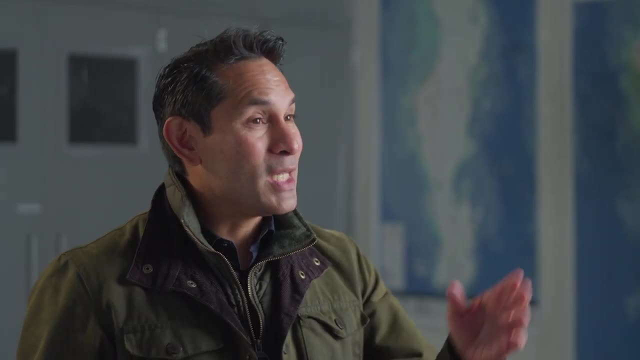 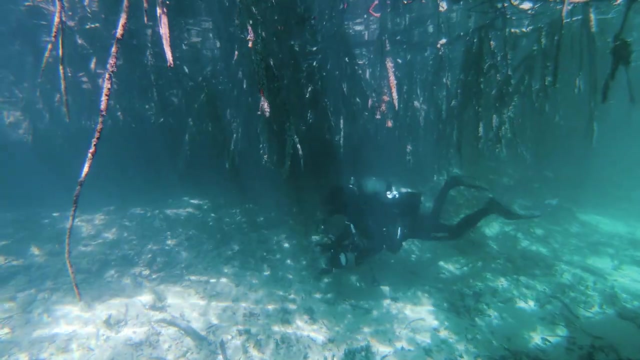 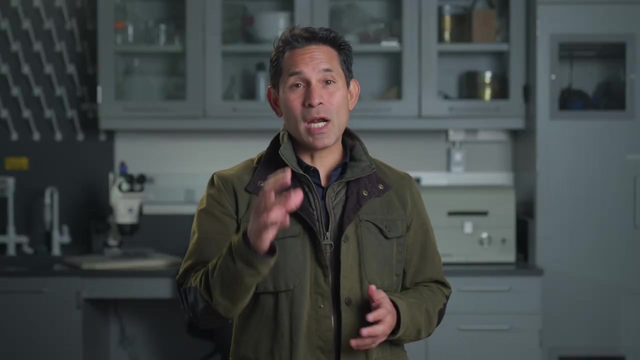 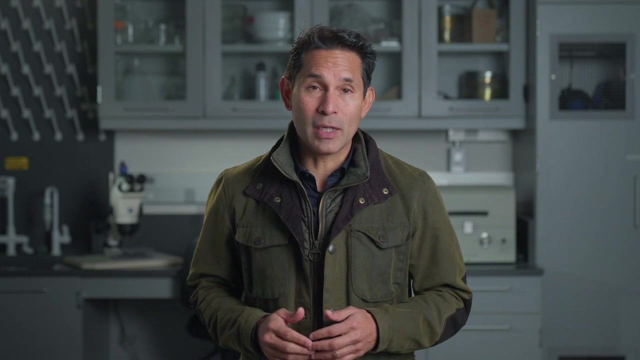 Some mangroves are ancient ecosystems. These forests have been growing on top of themselves for more than 2,000 years, accumulating and storing massive amounts of carbon. However, there is a problem. We have been losing large amounts of mangroves in the last five decades. Fifty percent of these ecosystems have been lost so far, and now more than ever we have an urgent need to protect them. 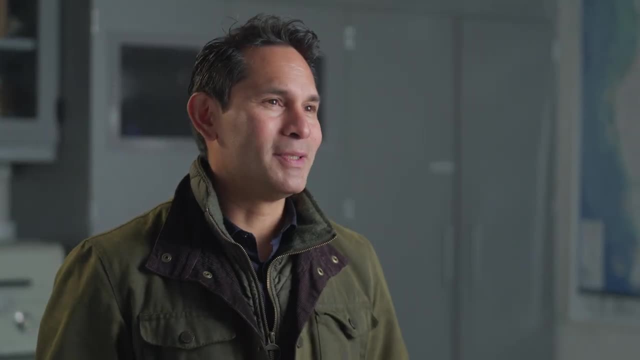 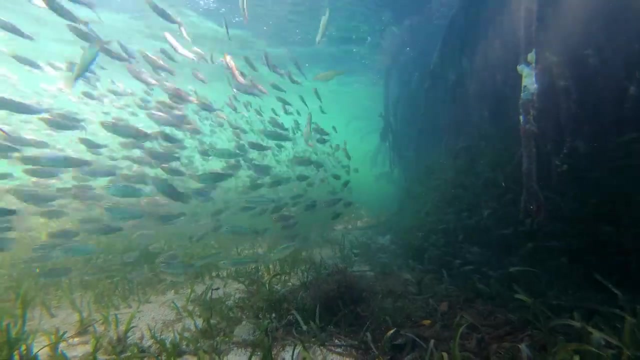 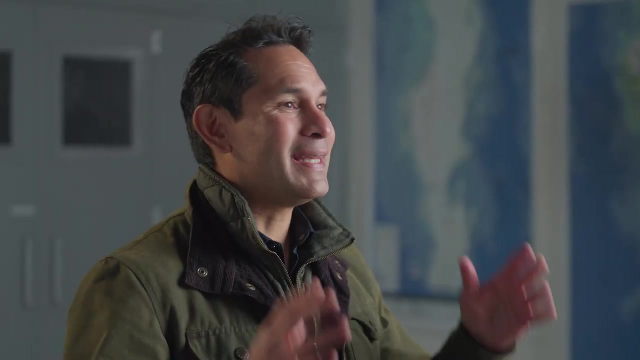 The first time I dove in a mangrove forest was unforgettable. I was able to see all the roots of the trees. I was impressed with this spectacular habitat for so many species and I was able to observe the mangroves. I was able to observe the habitat of a juvenile yellow snapper. We learned that the larger the mangrove forest, the more abundance of yellow snapper. Additionally, we were able to demonstrate that all other species show the same pattern. Since then I have been able to demonstrate these mangroves produce 11,000 tons of fishery products on an annual basis. for local communities That equal products worth almost 20 million dollars in the region. 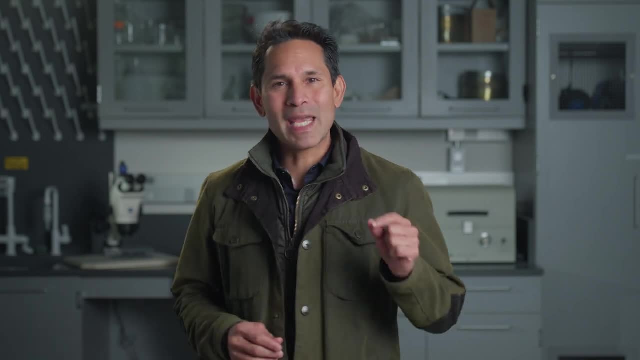 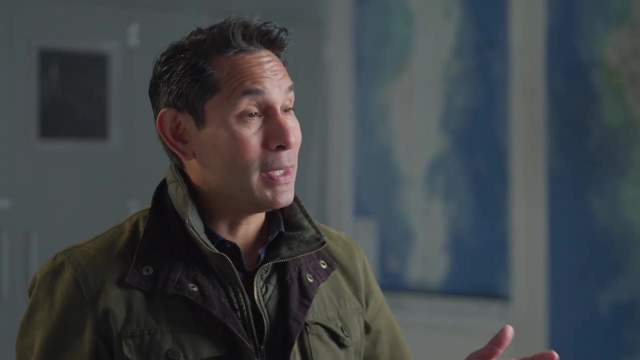 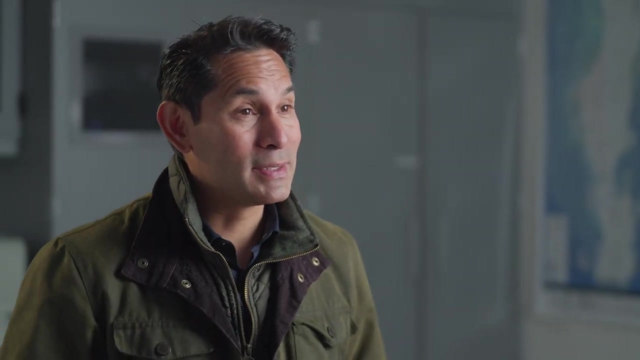 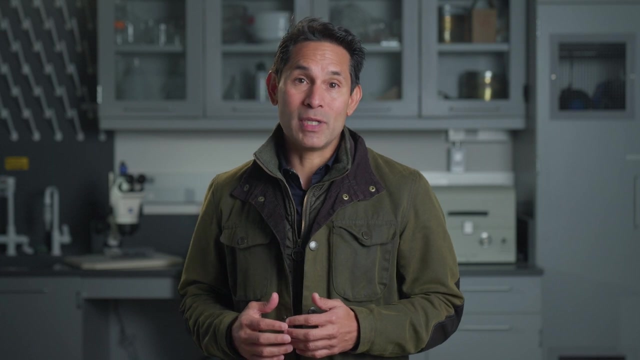 Just one hectare of mangrove every year produces around $37,500 in fishery products. We can quantify other services as well, like carbon sequestration. The organic material is captured in its root system and by different processes. Scientists can extract samples of sediments, study the samples and analyze how much carbon is being sequestered every year. 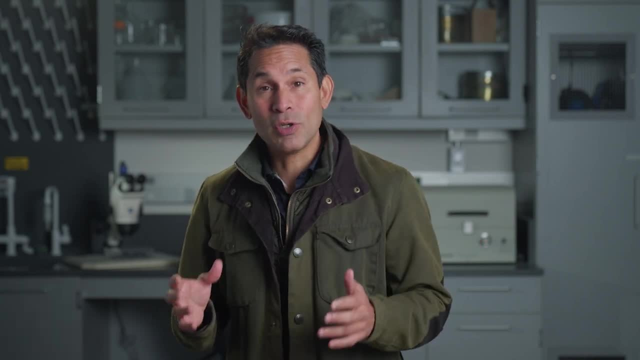 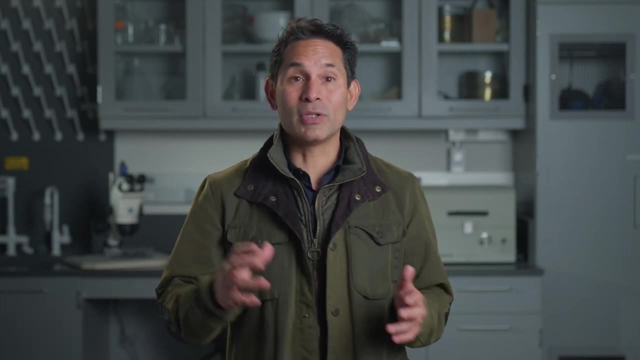 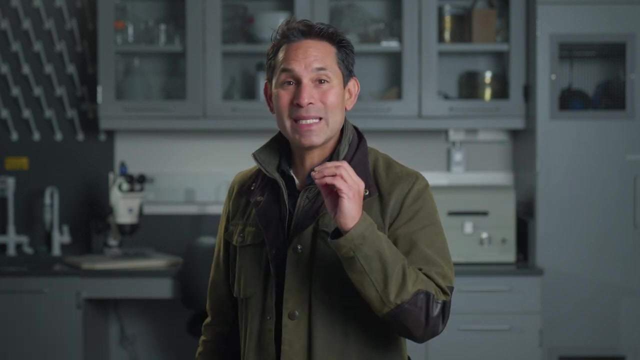 Estimating carbon and using the economic valuation of carbon sequestration, my research team has been able to show that Mexico should prioritize the conservation of different forests along the Mexican coast. In the same way that we estimate fisheries or carbon sequestration revenues, we can estimate the economic value of all the ecosystem services that mangroves provide to humans. 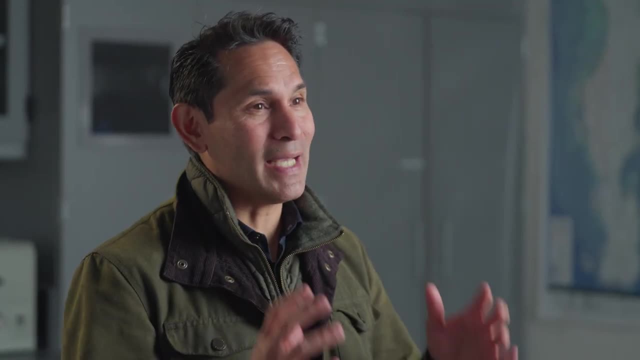 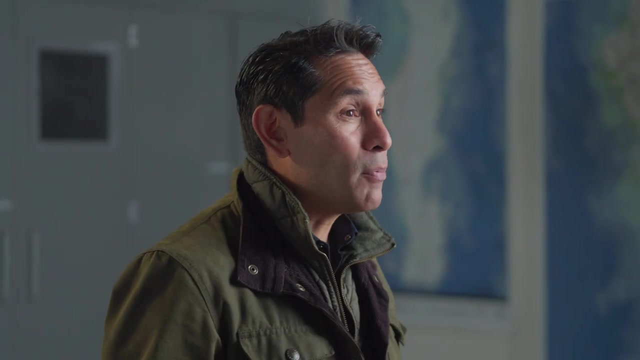 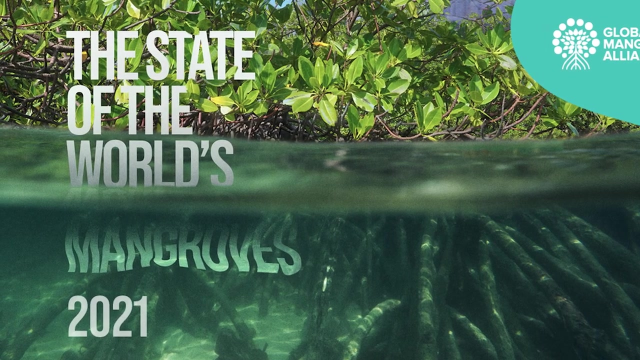 The United Nations has named mangroves as the superheroes in the fight against climate change, and many sustainability goals are based on mangrove protection. However, there are many barriers to reversing trends of mangrove deforestation. The 2021 State of the World's Mangrove Report shows that the rate of mangrove loss has declined. 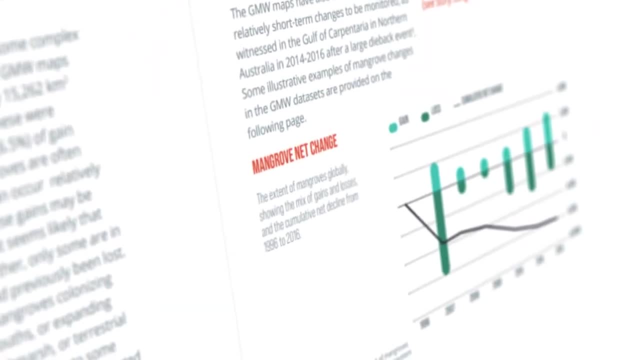 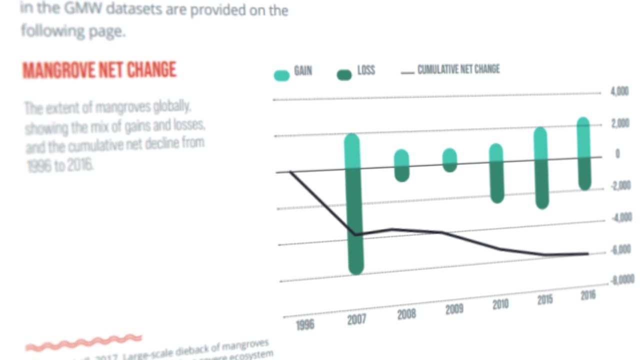 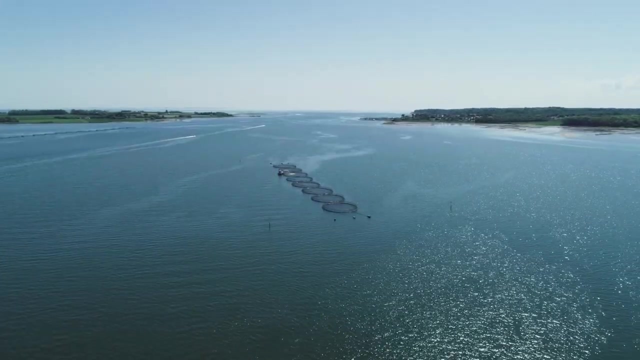 That means that in the 80s and the 90s, the speed at which we were losing mangroves was faster than today. Nevertheless, that doesn't mean that we are not losing mangroves. The drivers of this loss are the industrial activities: agriculture, aquaculture, the world's growing demand for palm oil for food and industrial products. 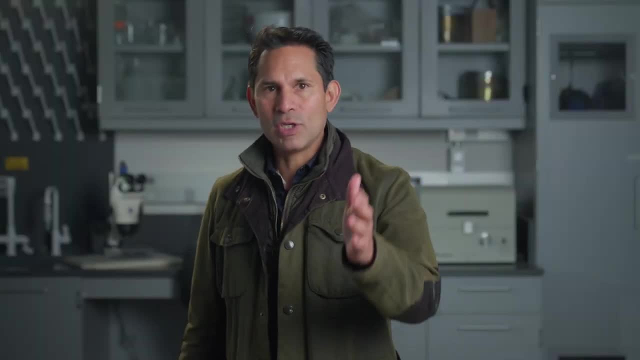 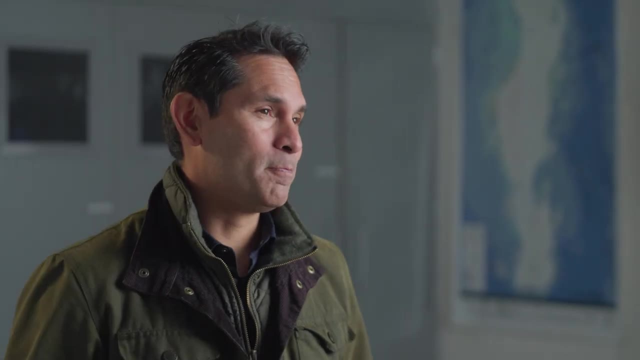 This demand is growing, especially in mangrove-rich countries like Indonesia and Malaysia. So how do we not only protect, but also restore mangroves around the world? My proposal is to introduce a model of solution-oriented science, rather than a model where scientists only decide. 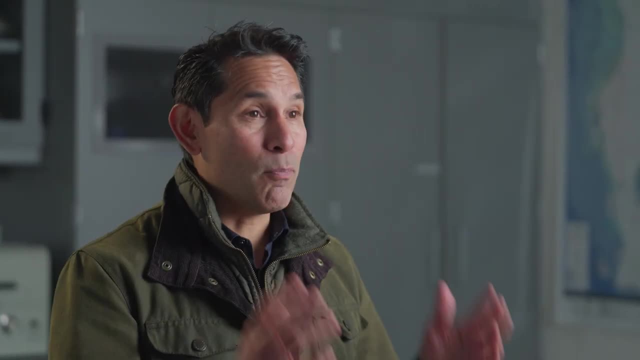 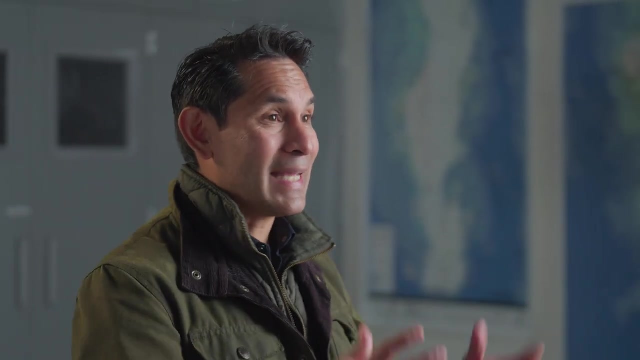 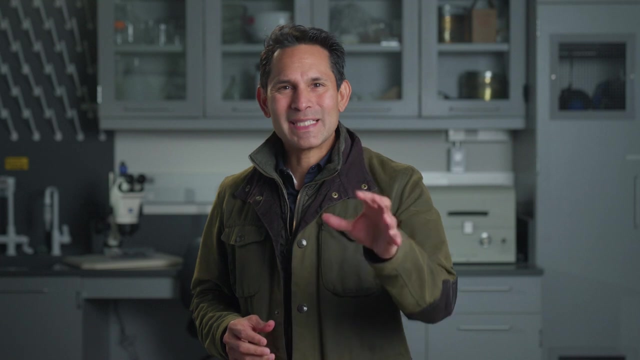 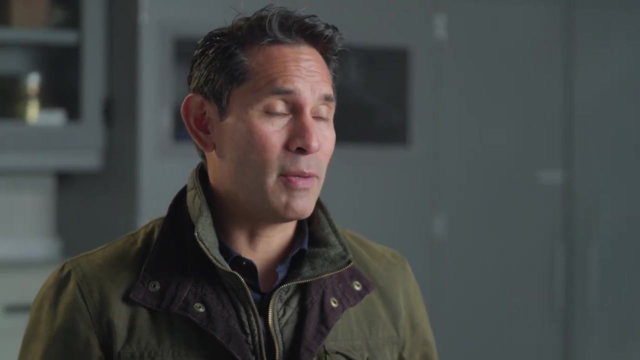 As scientists, we need to be a voice in the public arena. We need to be central to not just informing but organizing and enacting needed action plans. What I'm proposing is the first center for mangrove science diplomacy. We need scientists, their knowledge, their stories and their unique local efforts and experiences of protecting these extraordinary mangrove forests. 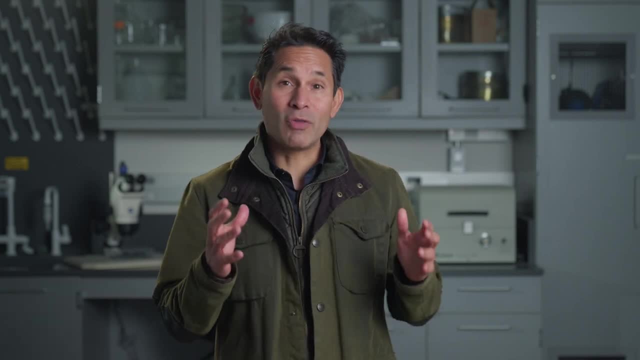 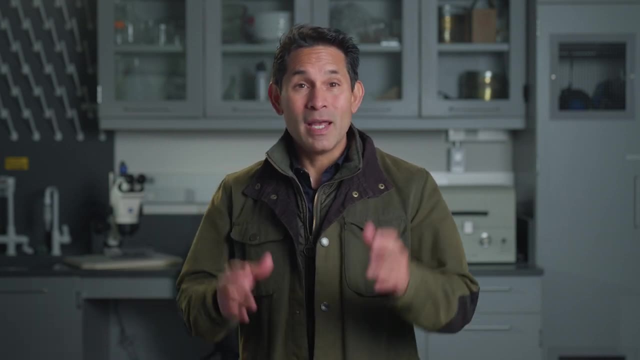 We need to find scientific leaders to help students. We need to stop mangrove deforestation collectively and to halt the trends that we have been seeing in the last 50 years. 13 countries in the world have 70% of mangrove cover. It's a small number of countries. This makes it possible to create a unique new network of scientists and a center to help with diplomacy to address mangrove habitat destruction. Scientists can help us address climate change. They can help with changing theories and also create a roadmap to protect mangroves. 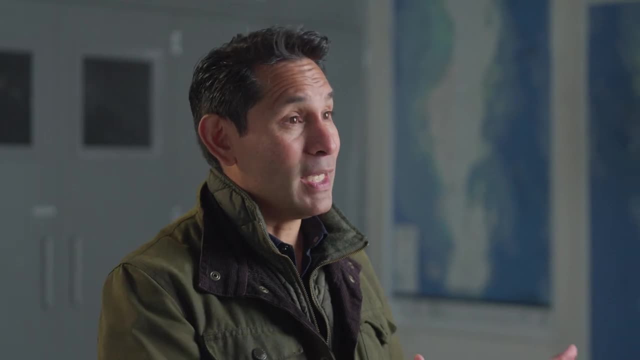 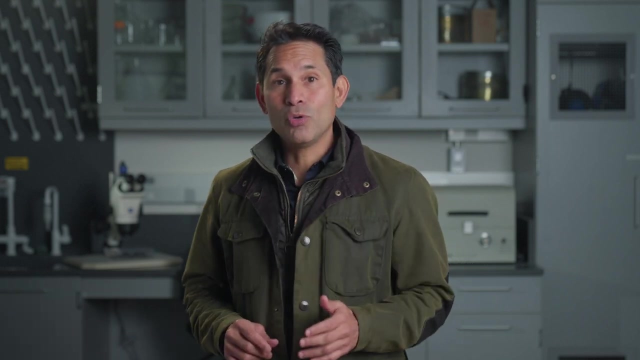 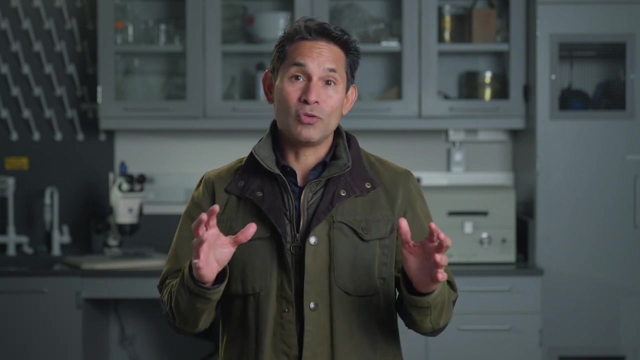 Scientists can be the ones that help create policy and produce solutions and outcomes, and not just provide the underlying data. If we are able to create a network of scientists and leaders across 13 countries, with 10 experts per country in 4 regions, we can create the first network designed to tackle the threats of mangrove deforestation.